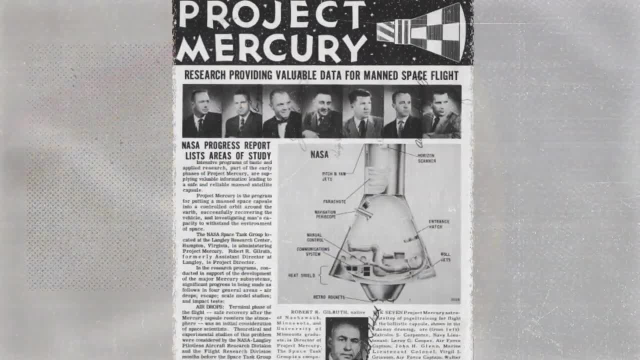 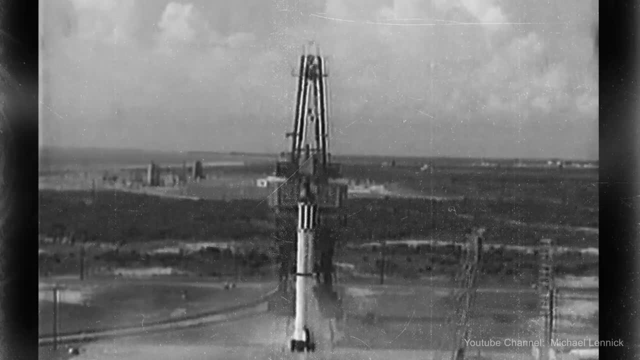 seriously in the old days was NASA. Project Mercury in 1958 signified the beginning of the space race. In its five years of existence, Mercury launched America's first satellite and sent Alan Shepard into space- The first satellite to launch into space. The first satellite to launch into space. 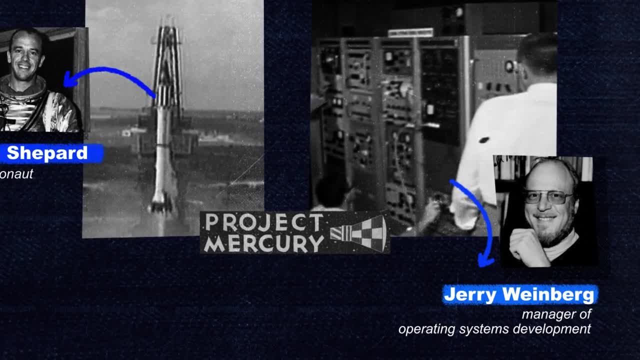 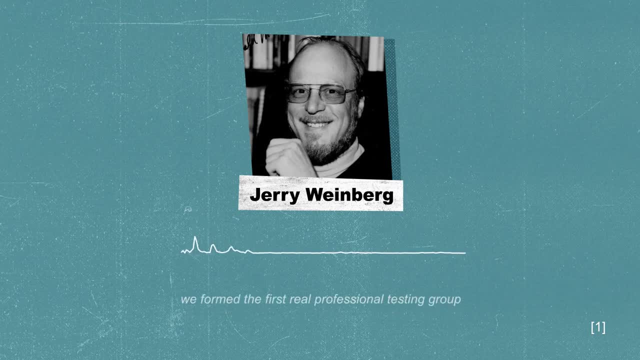 On starboard application. Many asked about it. Y2K was always considering software operations for the project and didn't have the typical attitude to testing. In a sense he was ahead of his own time. So we formed, as far as I know, the first real professional testing group that had. 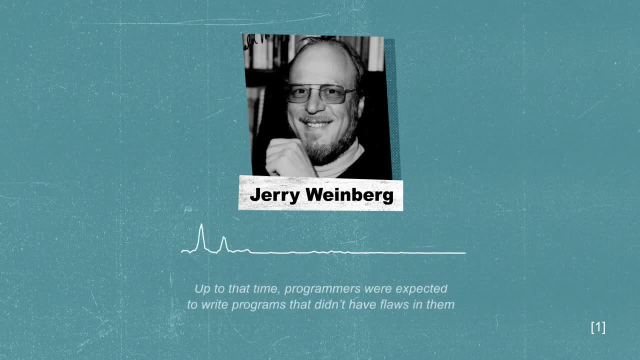 existed Up to that time, programmers were expected to – well, first of all, they were expected to be writing programs that didn't have flaws with them, And we were able to find the ones that did. もう, We made the first장, nory's testing. 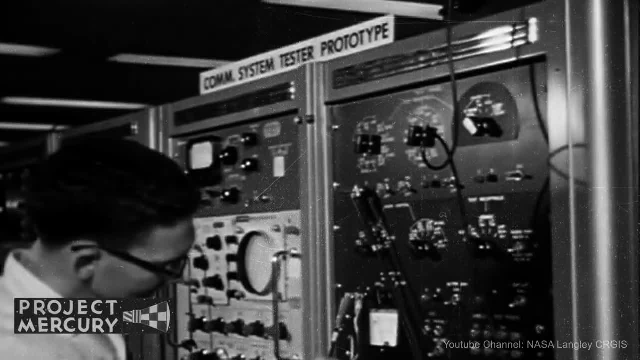 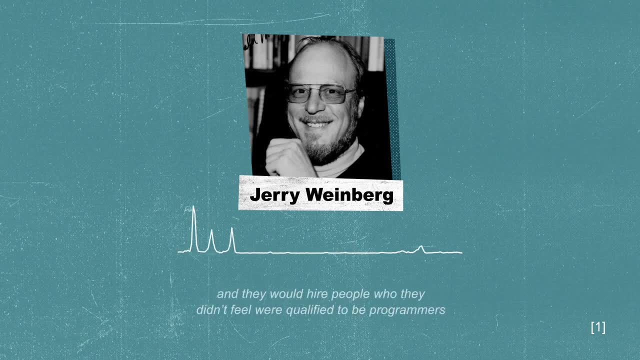 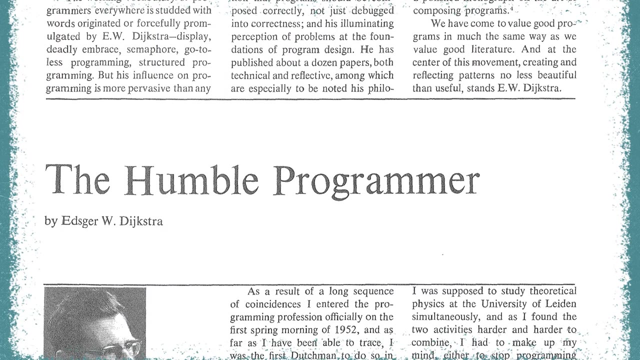 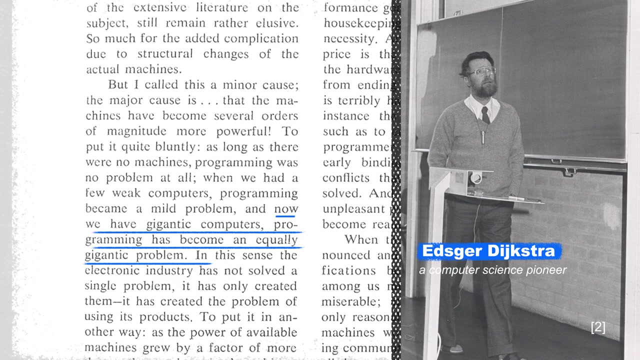 crew set the standard And the industry caught up, but not in the way it was intended. In the words of a computer science pioneer, Edgar Dijkstra, the industry scaled too quickly. At the dawn of software development, back in the 40s and 50s, software was built by those. 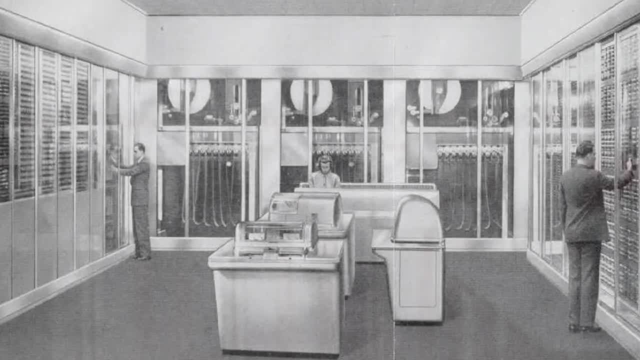 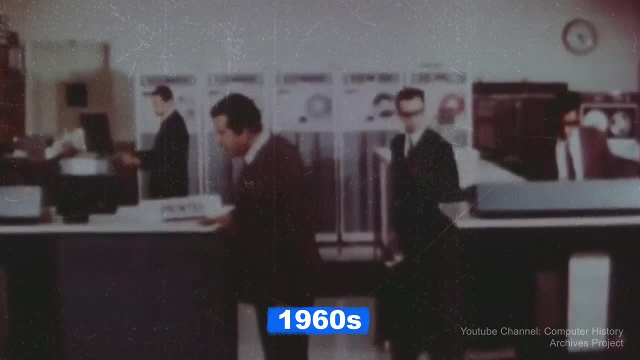 who would end up using it and on the machines that would run the program. but that was before engineering was commercialized. In the 1960s, IBM introduced System 360, a legendary mainframe computer built specifically to be modular and compatible with any task. 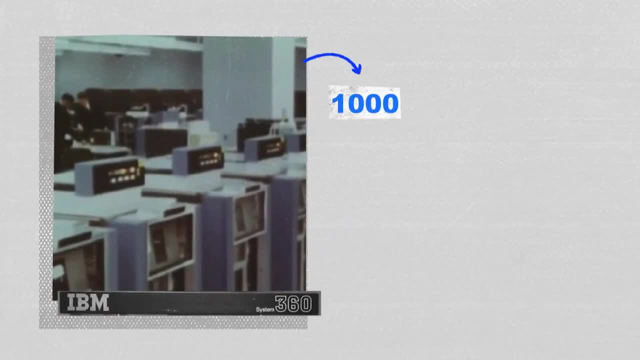 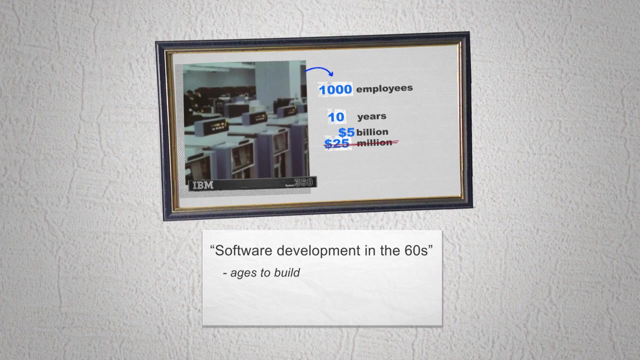 The cost and time it took to build were just as legendary. Around a thousand employees worked on the system for ten years and the initial budget of $25 million was raised to $5 billion. Ages to build. Companies hired excessive numbers of engineers to speed up development, but the pool of qualified 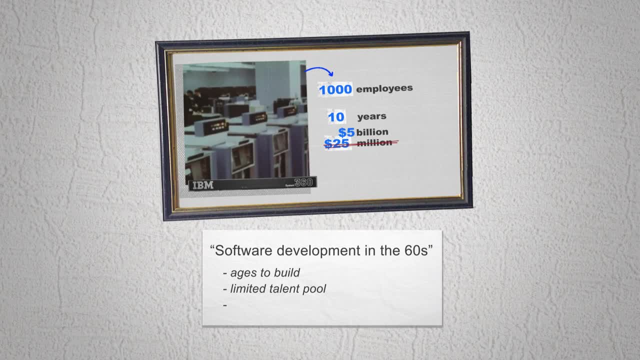 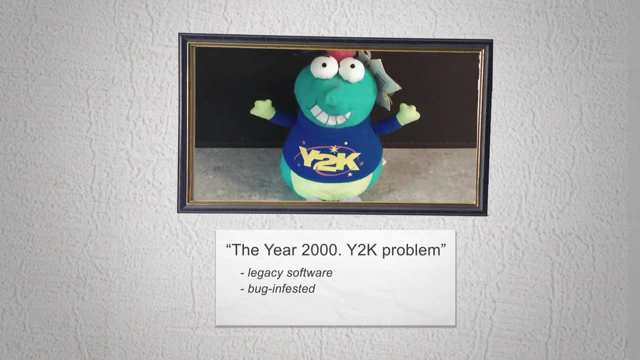 programmers was limited and soon they ended up with low-quality, bug-infested software. This was also the reason why 2K happened in the first place. People were still using legacy software developed decades ago by people who were unconcerned about the distant future. 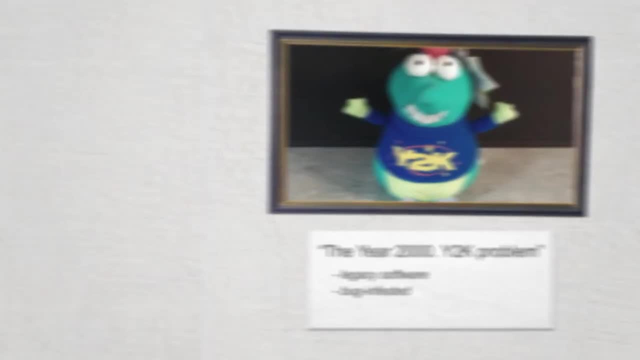 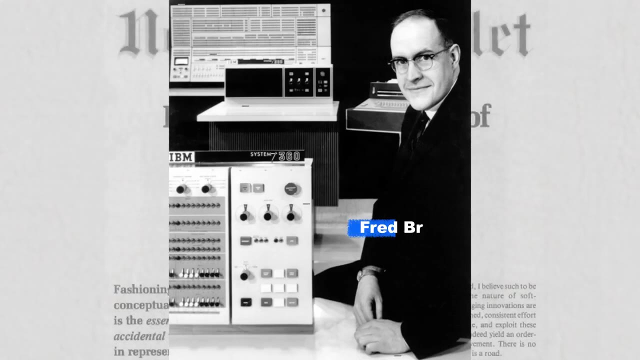 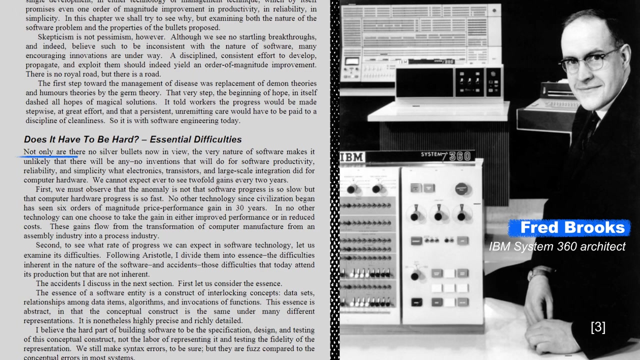 Solving the crisis was on the minds of developers and researchers until the 90s. In his famous article No Silver Bullet- IBM System 360 architect Fred Brooks lamented how the growing complexity of computer hardware was disproportionate to engineering practices. Not only are there no silver bullets now in view, the very nature of software makes it. 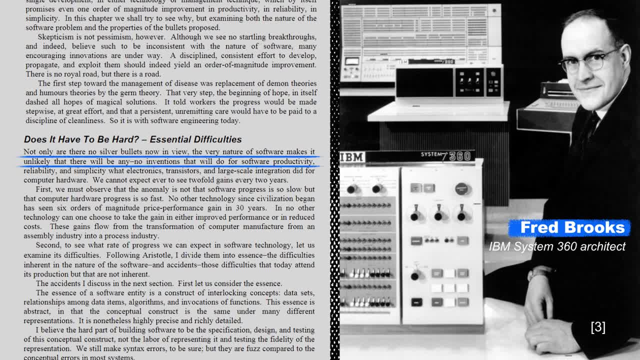 unlikely that there will be any. No inventions that will do for software productivity, reliability and simplicity, with electronics, transistors and large-scale integration did for computer hardware. We cannot expect ever to see two-fold gains every two years. It was like a dream. 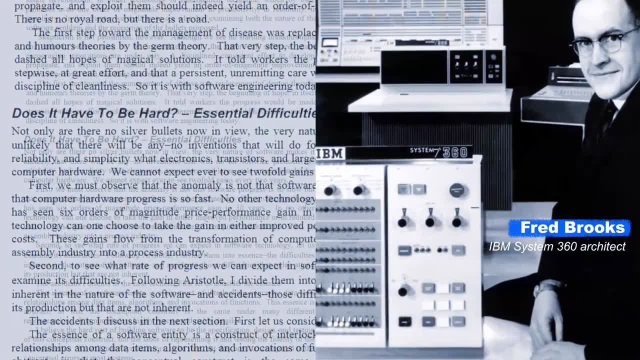 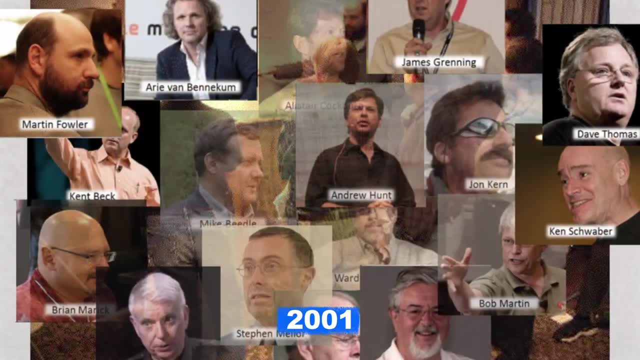 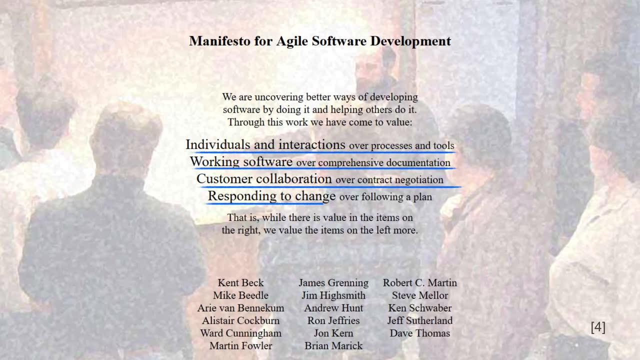 It was like a dream. It was like a dream And software development had nowhere to grow. Turns out, he was wrong. In 2001, 17 software development leaders created the manifesto for agile software development. This new approach was a direct response to the traditional method known as waterfall. 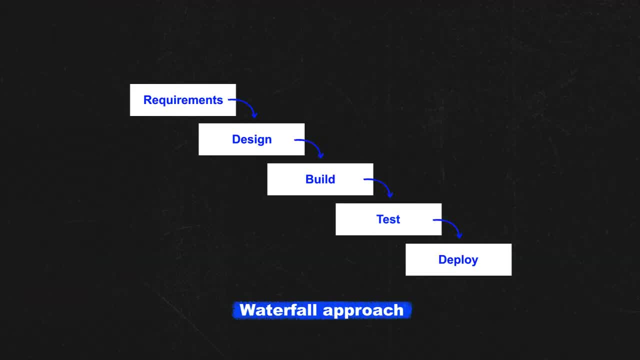 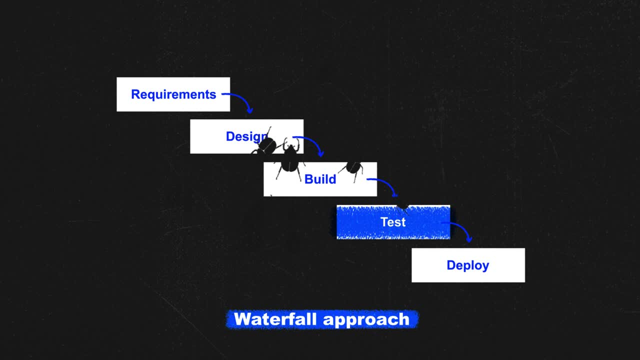 that migrated from the old manufacturing practices In Waterfall. you work in stages that strictly follow one another, which is intuitive but risky If, or more correctly, when a test is performed. If a tester finds a bug in the code, design or even product requirements, the project has to start all over again. 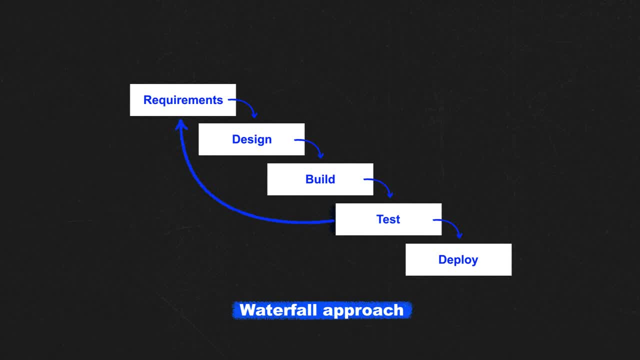 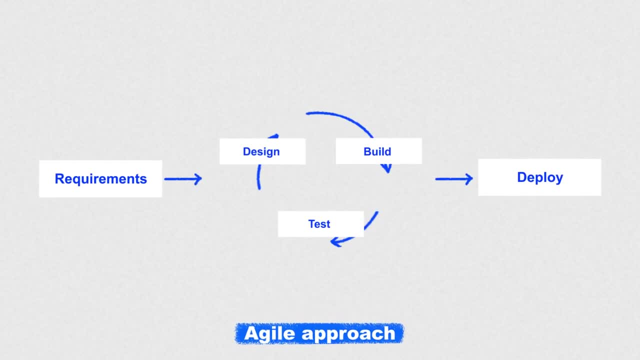 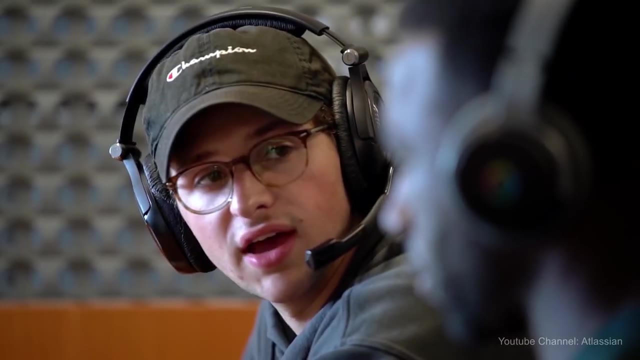 This also means that the engineering and testing teams don't work closely together. Agile's 12 principles all come down to a few core ideas: Embrace change, stick to the shorter cycle and collaborate more. Yes, open space offices likely became a trend due to Agile recommendations. 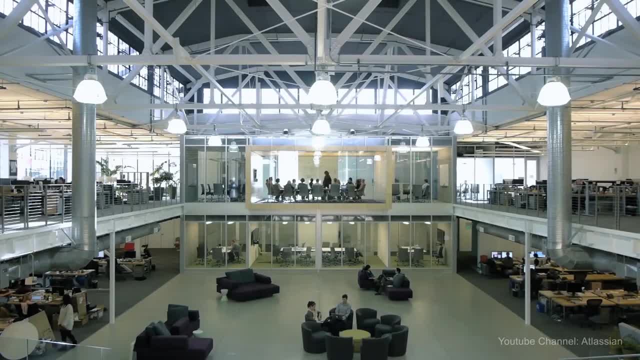 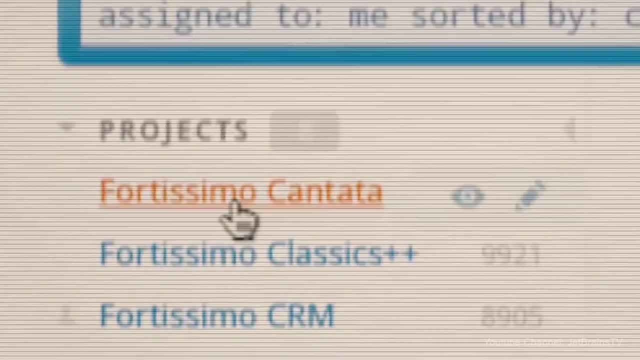 Testers are now the required members of the engineering team who maintain the product quality from the very start. Now, feedback exchange is instant and bug fixes happen at the time of coding. Also, automated tests are way more widespread. Testing became more than a routine task of sorting through the code. 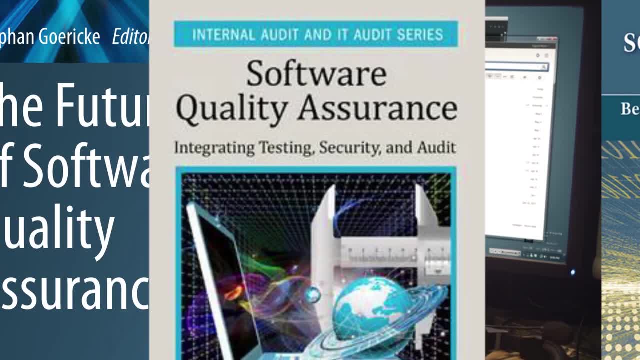 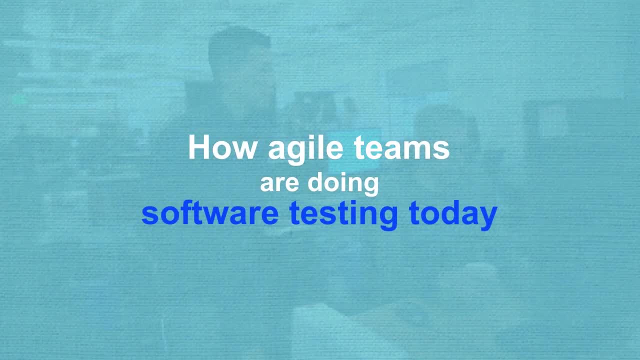 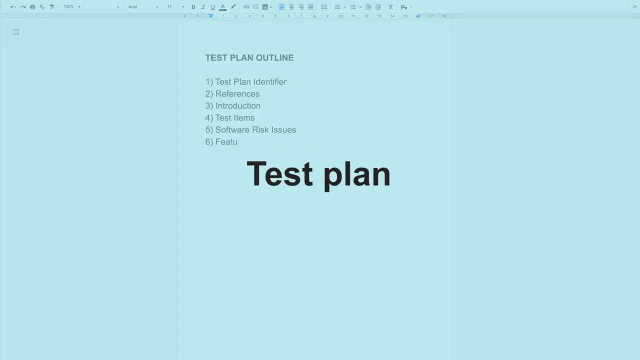 A new process deserved the title of Quality Assurance, which also covers planning, monitoring and control. Here's how Agile teams are doing software testing. today, Planning is something considered very important. It's considered anti-Agile. Here's an approximate list of things that should be recorded in a test plan. 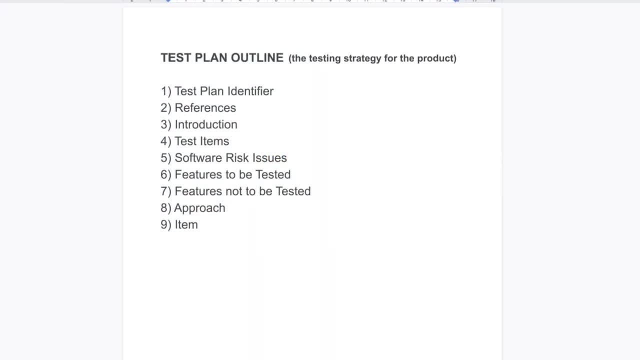 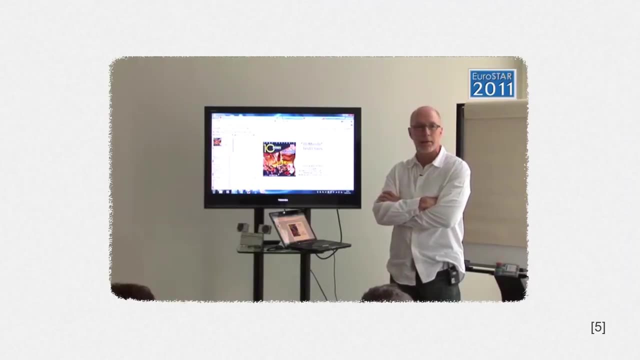 a document dictating the testing strategy for the product, But Agile test leaders are looking into simpler alternatives, And test plans were one of the things that were really annoying me about Google. They annoyed me at Microsoft, too. They've annoyed me. They've always annoyed me. 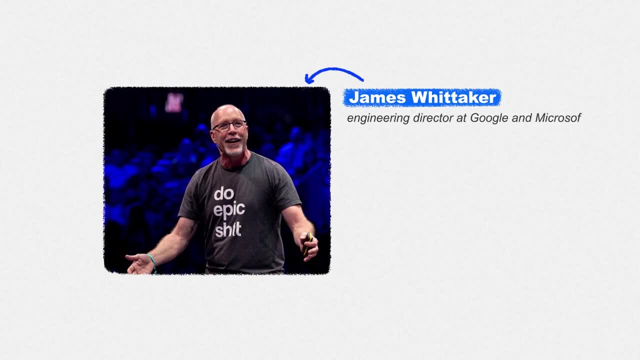 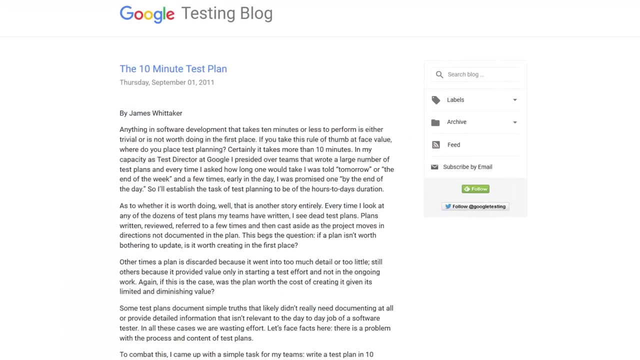 This is James Whittaker, former engineering director at Google and Microsoft and author of How Google Tests Software. He came up with a hugely popular technique for writing tests. It's called test documentation, called the 10-minute test plan. James defined three core elements that a test plan needs. 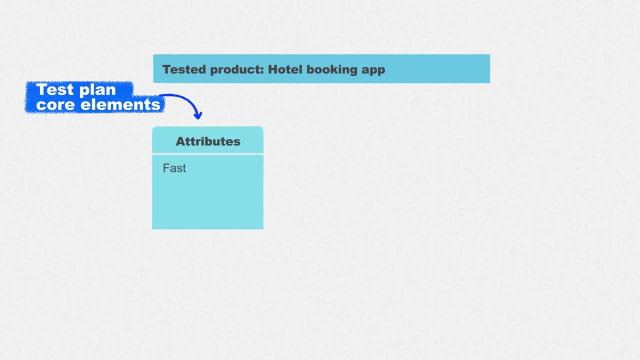 First are the attributes. These are the adjectives describing the main purpose of testing. What is testing supposed to check? Then the components: What are we testing? These are the nouns describing pieces of code or features. Finally, we document capabilities. 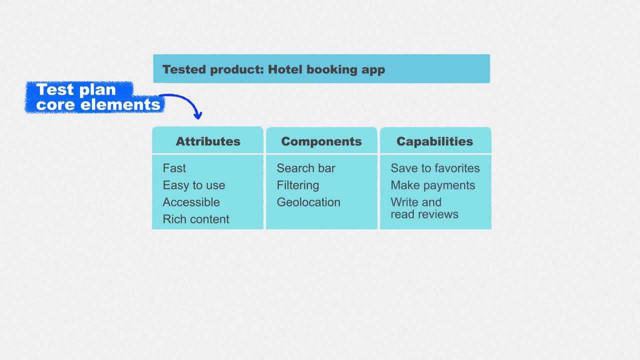 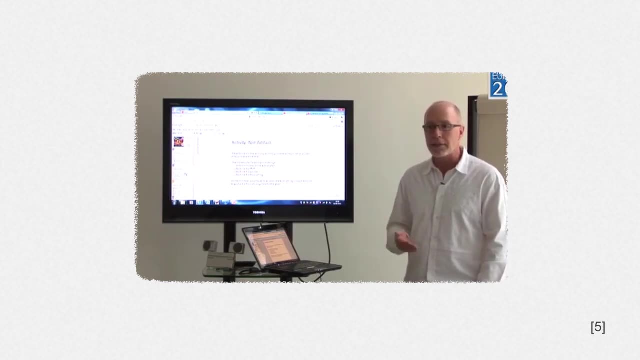 Here you use verbs to explain what a user should be able to do, And we never built a test plan in 10 minutes, but we did do. We did discover the things that are absolutely important in a test plan and we threw away the rest. 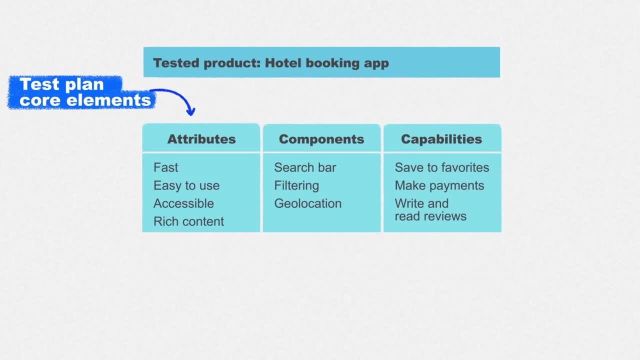 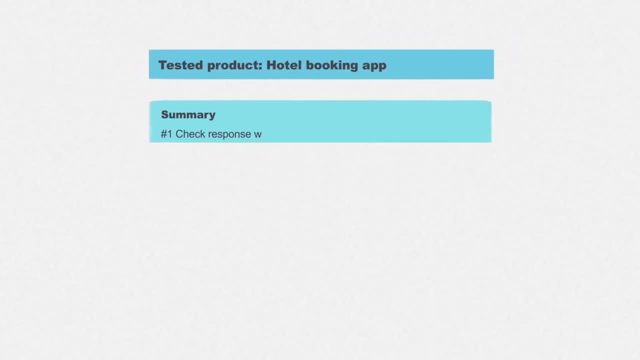 Even the minimalistic version of a test plan will be enough to start a second stage, which is writing test cases and test scripts. A test case is a detailed description of the task that would allow you to perform the test and then determine if the program passed or failed. 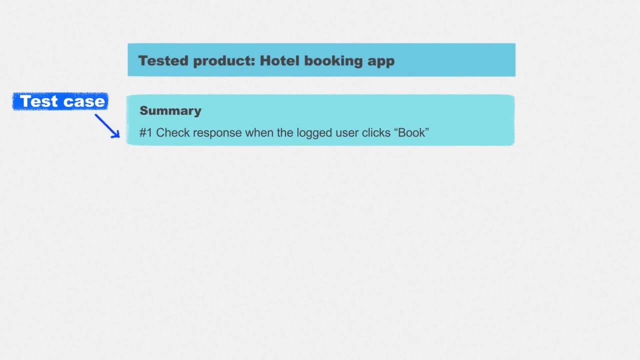 Say your task is to check what happens when a logged user tries to book a hotel room. The test case will have information about the steps you'll need to take, conditions that must be followed before you do the test and the expected outcome. This would actually be an example of functional testing. 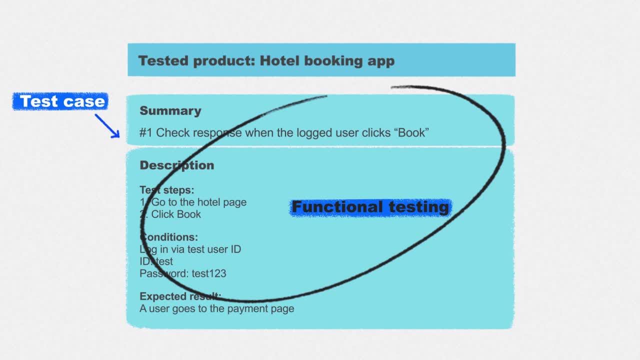 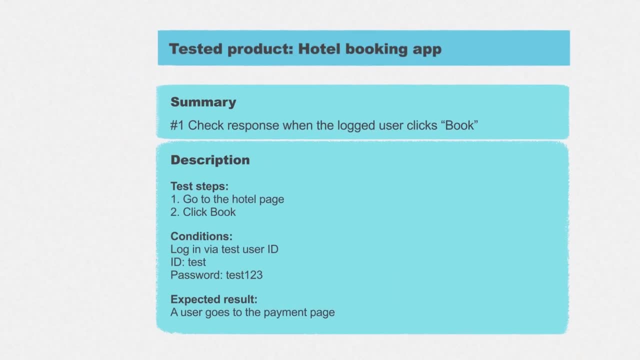 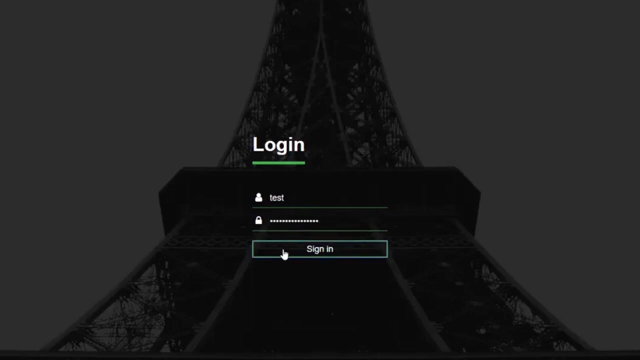 a type of test performed when we want to check how the software works in terms of features. There are a few types of tests to know about. Functional testing usually has an input- what to do- and an output- what we should expect. This testing can be done even by people who have minimal knowledge. 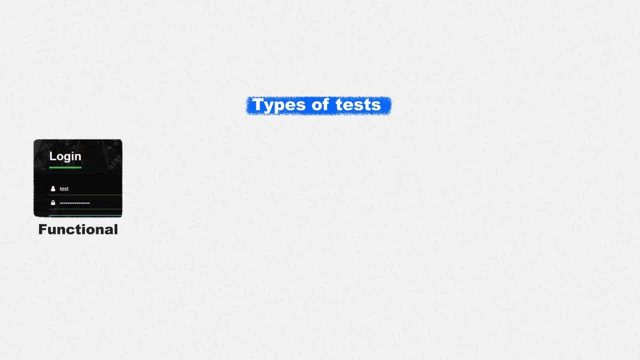 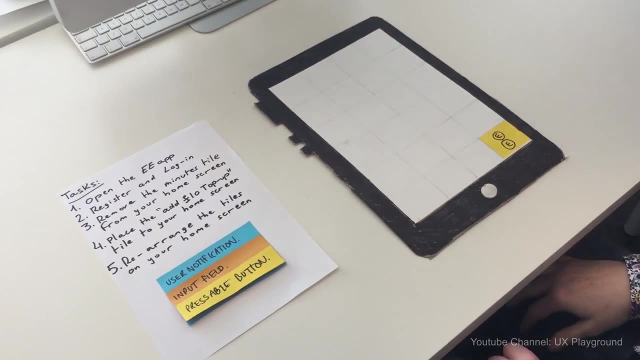 about how the system works from the inside, which is why it's also called black box testing. What else could you test using a black box approach? Usability, for example? You don't have to read code to understand if the system is easy to use. 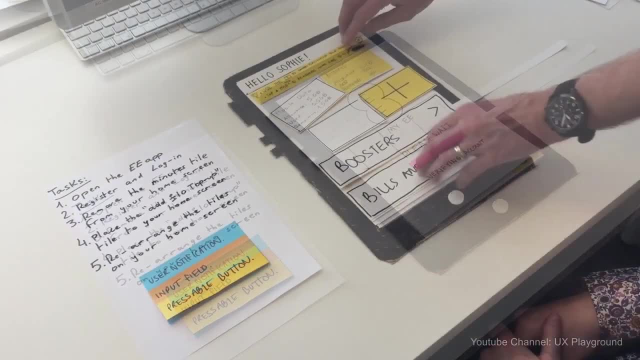 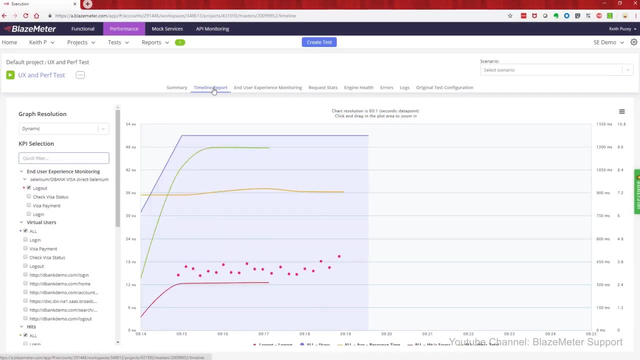 There's also use case testing, when you have to check if the software will be used as intended. This would verify the work of UX designers. Black box testing will also be enough to check the system's stability and performance, basically the conditions under which it would or wouldn't crash. 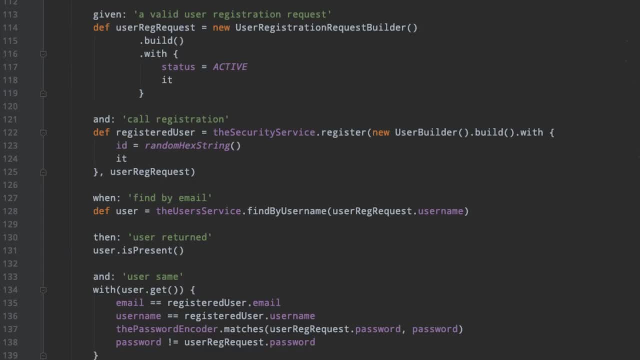 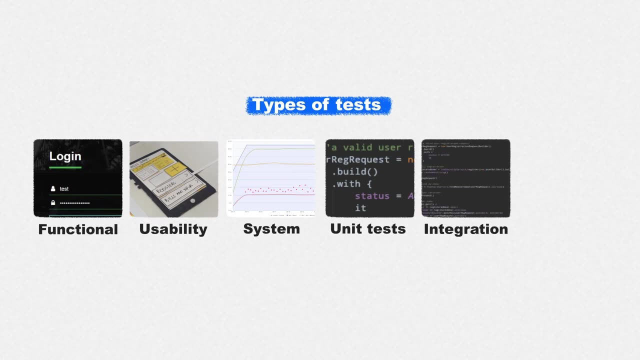 But often you need to test the quality of the code itself and its security, how its smallest parts work and how these parts work together. This is called white box testing, and it's either done by programmers who develop this particular software or test engineers who know how to code. 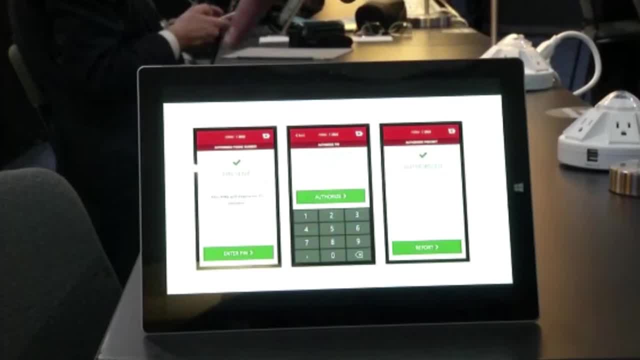 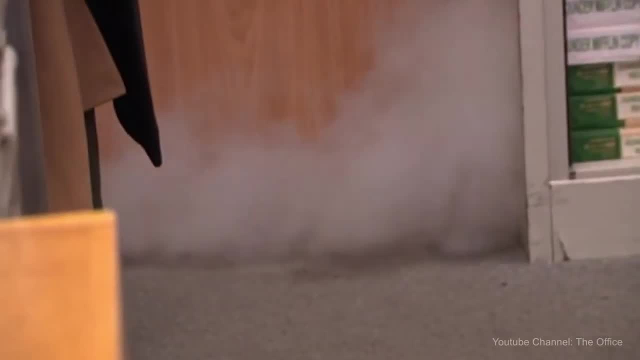 Not all tests need written cases. Sometimes tests are done sporadically to save time or simply to see what will happen if we improvise. This is called ad hoc testing like a fire drill. Obviously, this should be done by a human tester. 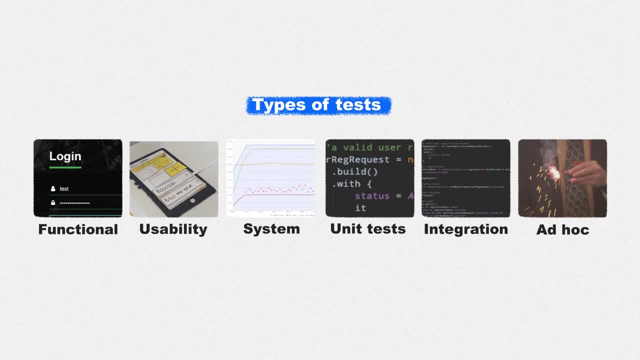 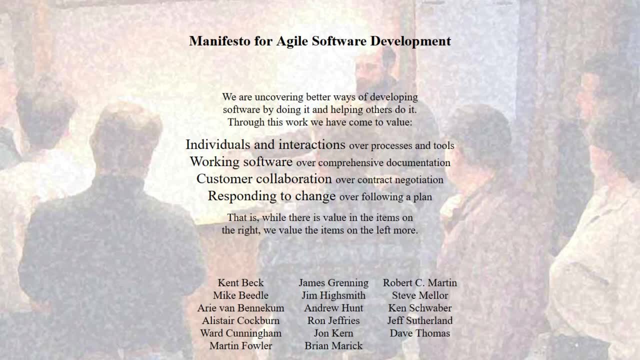 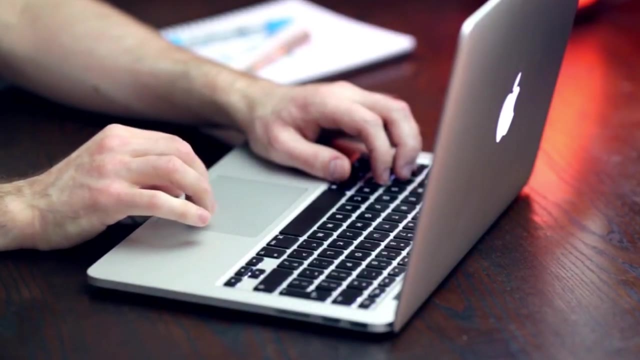 because the machine can't improvise like a human. But what can a machine do? The hits and misses of automated testing. Before the Agile manifesto emerged, test automation was a badly underused technique, But it makes perfect sense in the logic of continuous iterative improvement. 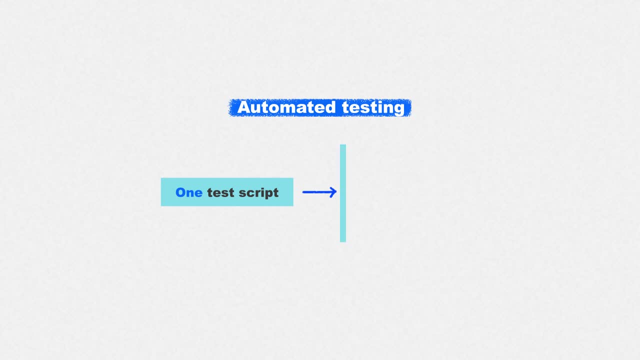 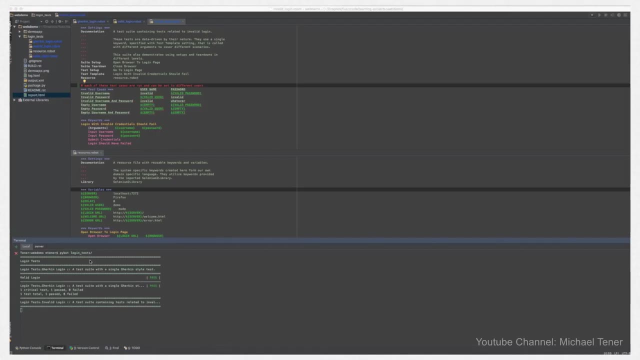 You write a test script once and run it simultaneously on as many devices or browsers as you want, as many times as you want and for as long as you can leave your computer on. Here's an example of an automated test checking system. This is an automated test checking system. 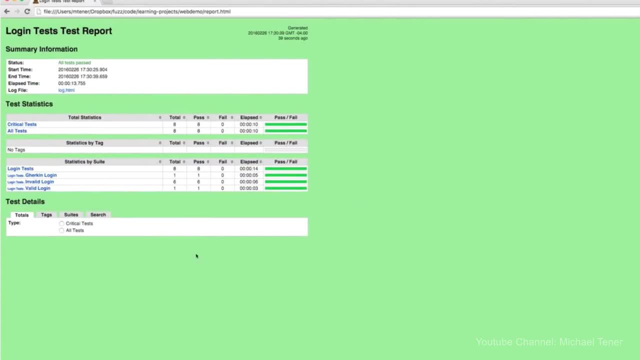 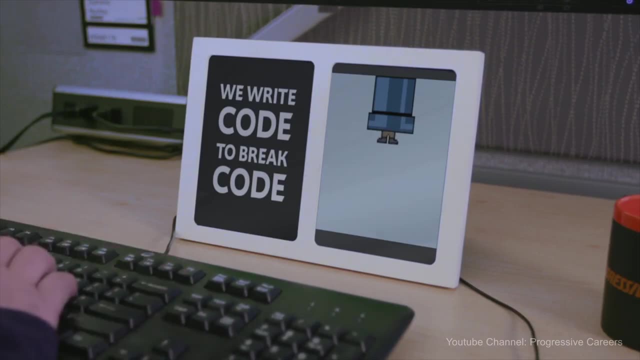 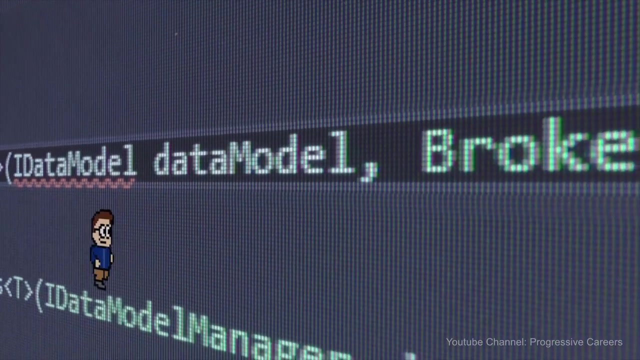 that uses a system response to invalid logins, And here are the reports it made. Using it, however, can be challenging. Only highly skilled testers can write test scripts, so project managers have to be smart when distributing testing efforts, While a machine can't be trusted with all tests. 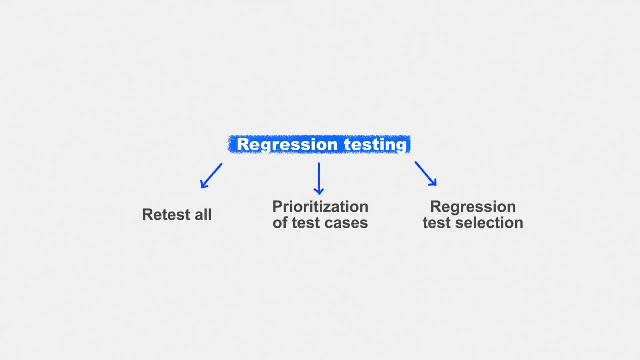 in some situations it's a real lifesaver In regression testing, for example. regression testing aims to check how the system works after changes. It's even totally unfair to make people perform dozens of the same tests every time you want to ship an update. 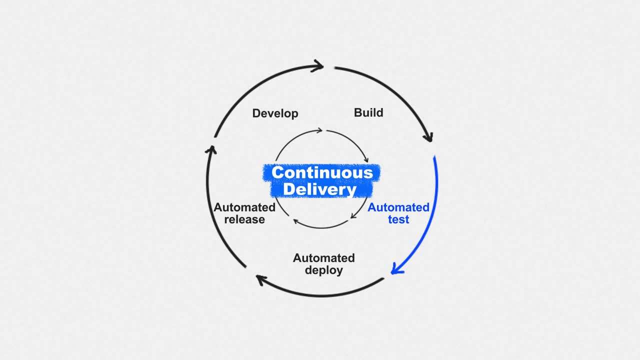 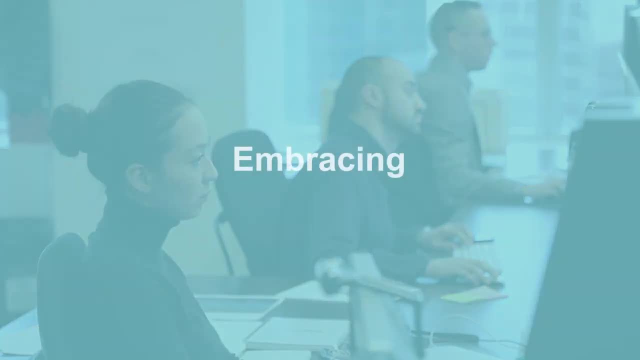 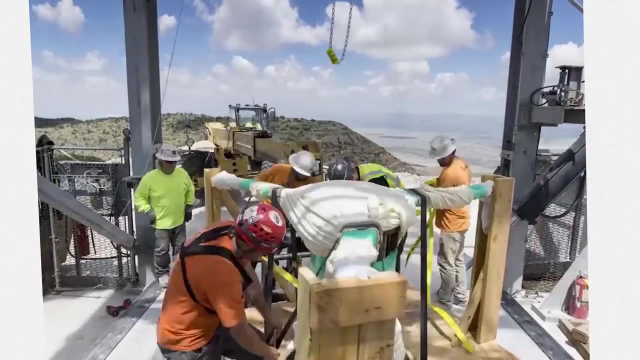 Automation testing is also one of the pillars of continuous delivery. the new stage in the evolution of Agile DevOps practices are also dependent on continuous testing, Embracing the long-term thinking. There's a monumental mechanical clock being built in the San Diablo mountain range of West Texas right now.